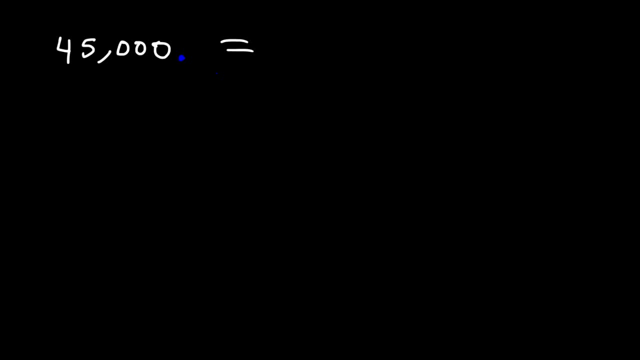 Now you want to move the decimal in between the first two numbers, that is, between the 4 and 5.. So I'm going to move it 4 units to the left: 1, 2, 3, 4.. 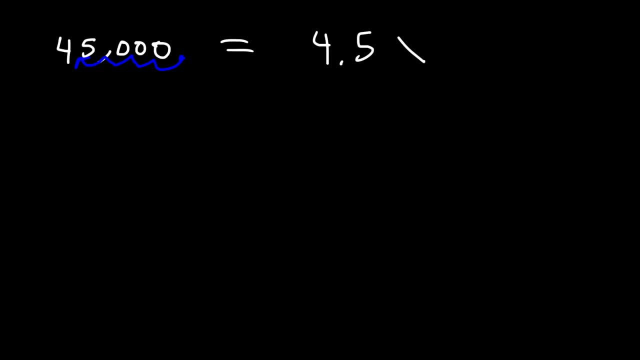 So 45,000 is equal to 4.5 times 10 to the 4.. Now it's important to understand that if this number is positive, it's associated with a very large number. If this is a negative exponent, it will be associated with a very small number, a number between 0 and 1.. 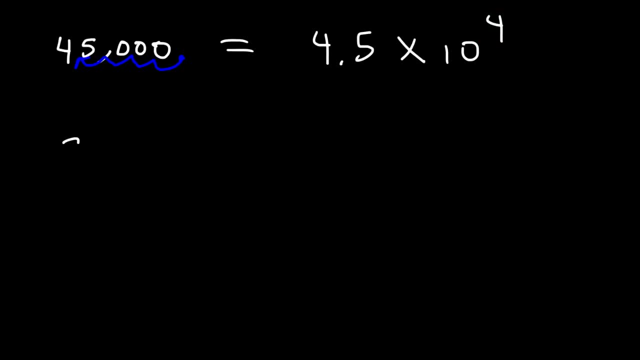 So let's work on some more examples. Try these two examples- Actually maybe more than two: Let's say 3750, 580,000, 72,000,000, and let's say 9.3 billion. 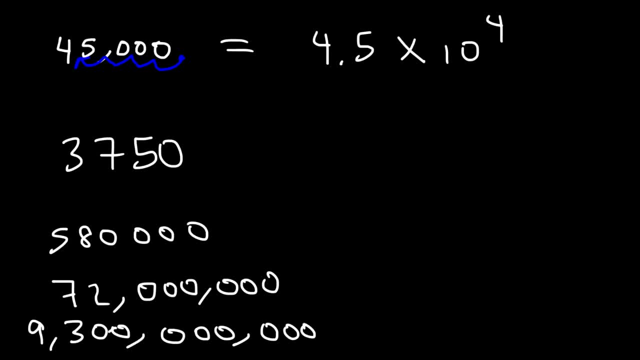 Go ahead and convert these numbers into scientific notation. Feel free to pause the video, So let's start with this one. I'm going to put the decimal between the 3 and the 7.. So this is 1,, 2,, 3.. 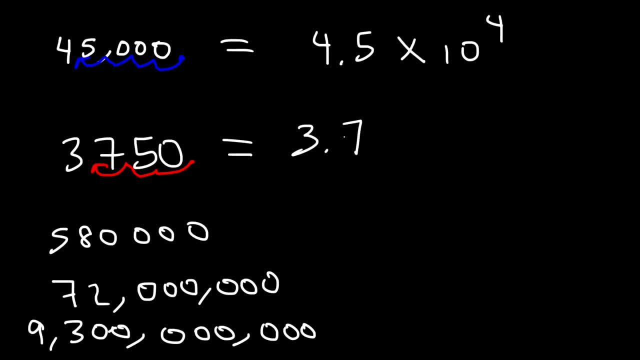 Since I moved it three spaces to the left, this is going to be 3.75 times 10 to the 3rd power, And that's pretty straightforward. Now let's move on to the next one. So I want the decimal point to be between the 5 and the 8.. 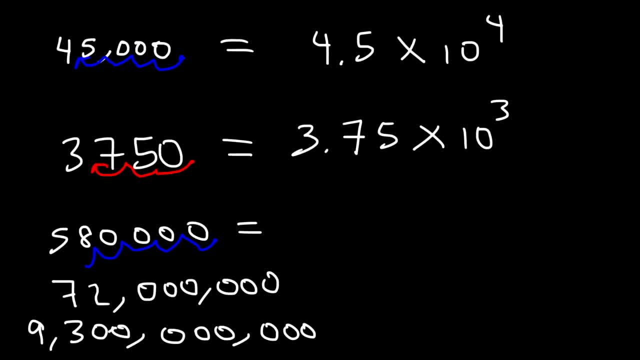 So I'm going to move it 1,, 2,, 3,, 4, 5 units to the left. So therefore, this is going to be 3.75.. So this is going to be 5.8 times 10 to the 5.. 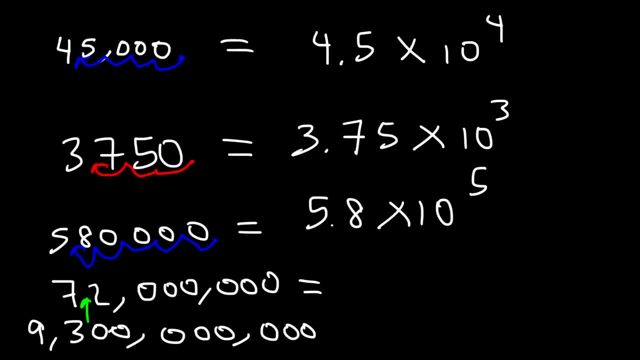 Now for the next example. I want it to be between the 7 and the 2.. So this is going to be: this is 3,, 6, and then 7.. So I moved it seven spaces to the left. 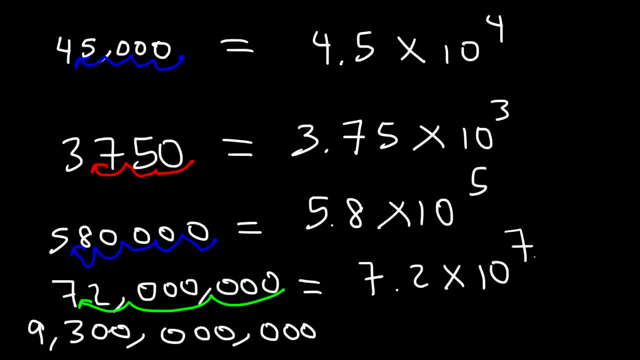 So it's going to be 7.2 times 10 to the 7.. And that's it for that one. Now for the last one. I'm going to start here: 3.. 6,, 9 units to the left. 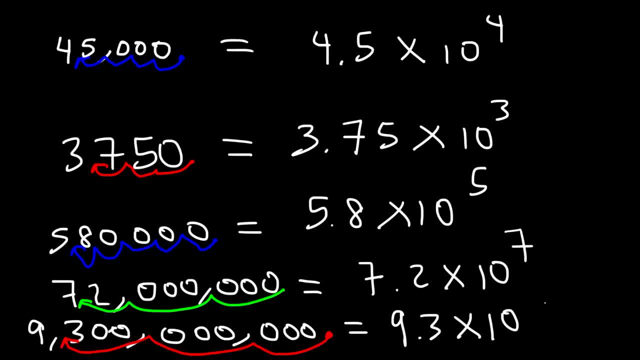 So this is going to be 9.3 times 10 to the 9th power, And that's a simple way to express very large numbers using scientific notation. Now what about some small numbers, For example .0023.. 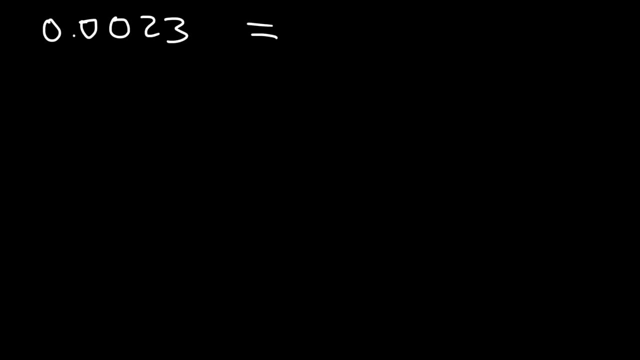 We still want the decimal to be between the 2 and the 3.. But this time I'm going to move it to the right as opposed to the left, So I need to move it three spaces to the right. So therefore, this is going to be 2.3 times 10 to the negative 3.. 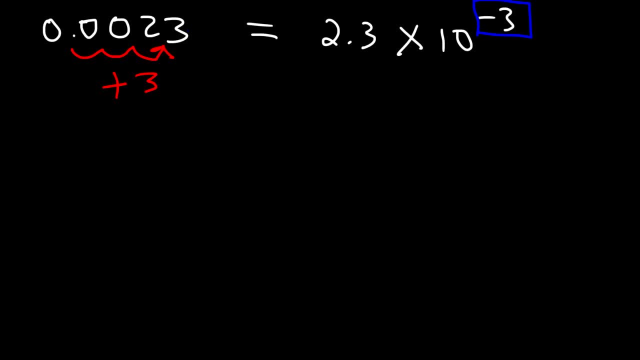 Now keep in mind: a negative exponent will always be associated with very small numbers. A positive exponent will be associated with very large numbers. Here's some more examples that you can try. So this is going to be 7.6 times 10 to the negative 4.. 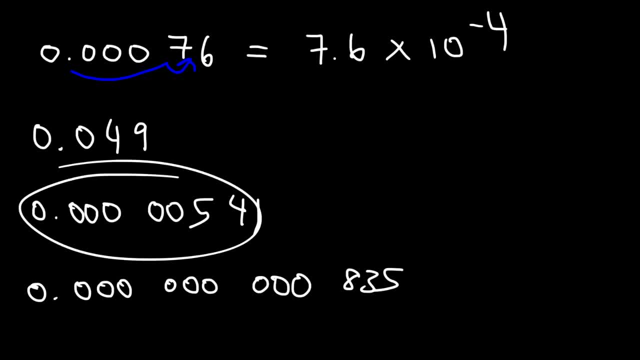 So anytime you have these decimal values, it's going to have a negative exponent associated with it. So this is going to be 7.6 times 10 to the negative 4.. So this is going to be 7.6 times 10 to the negative 4.. 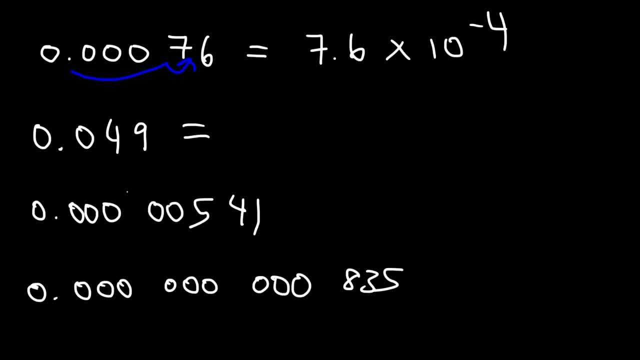 associated with the scientific notation number. So for this one I've got to move it two units to the right, and so that's going to be 4.9 times 10 to the minus 2.. Now for the third example. this is 3, 6, 7.. 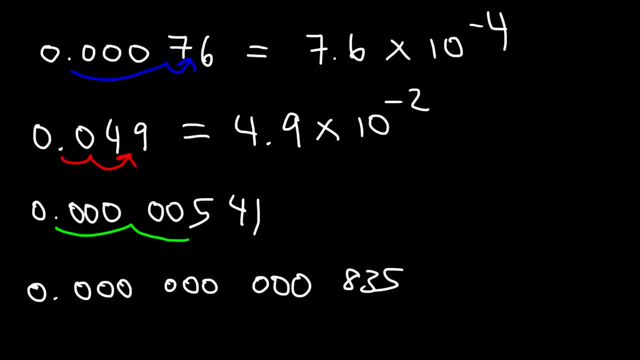 Actually not that far. I need it to be between the first two numbers, so 3 and 6.. So this is going to be 5.41 times 10 to the negative 6.. This is 3,, 6,, 9, and then 10 units to the right. 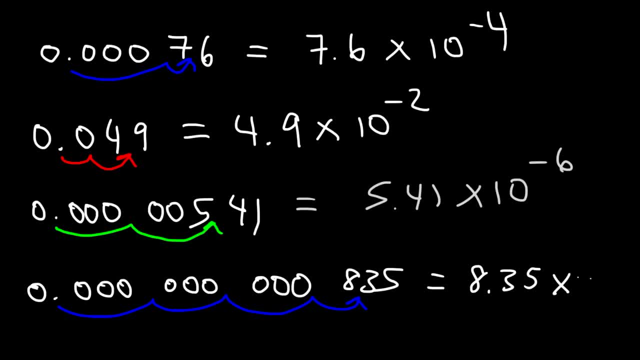 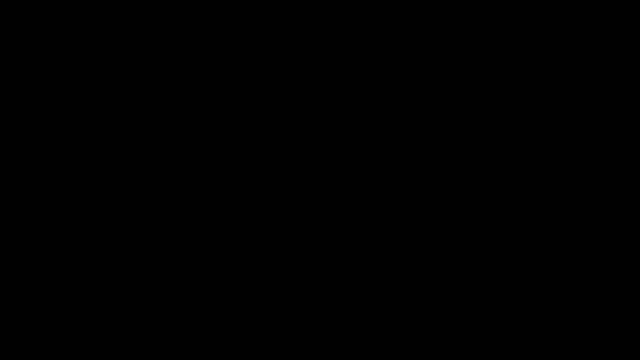 So this is going to equal 8.35 times 10 to the negative 10.. And so now you know how to convert a number in decimal notation or standard notation into scientific notation. Now let's switch it up a bit. Let's work on. 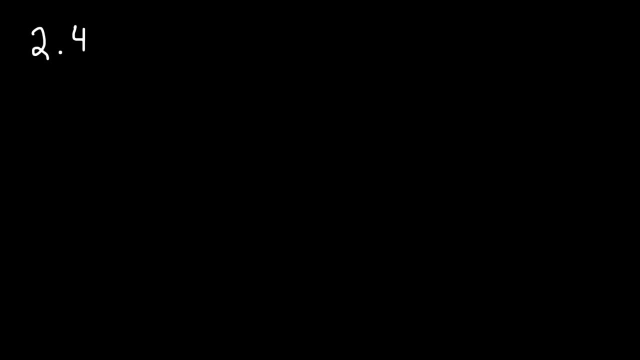 converting a number from scientific notation to standard notation. So let's say, if we have 2.4 times 10 to the 2. What is this equal to? Now keep in mind that we said that if we have a positive exponent, it will be associated. 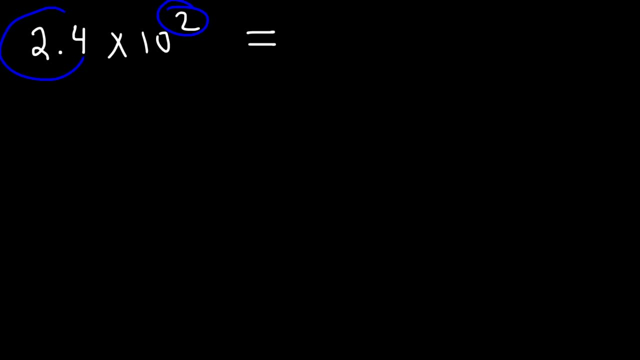 with a larger number. So we need to increase the value of 2.4.. So should we move the decimal to the right or to the left To increase the value? we need to move it to the right. So we have the number 2.4, and let's add some zeros to it. 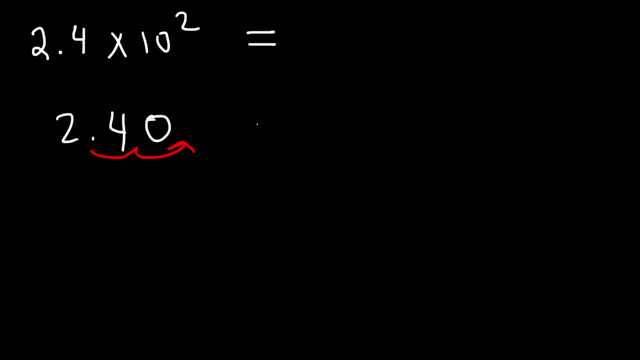 So we're going to move it 2 units to the right. So therefore, this is going to change to 240.. And that's the answer. Now, if you think about what this expression means, 10 squared that's 10 times 10, which. 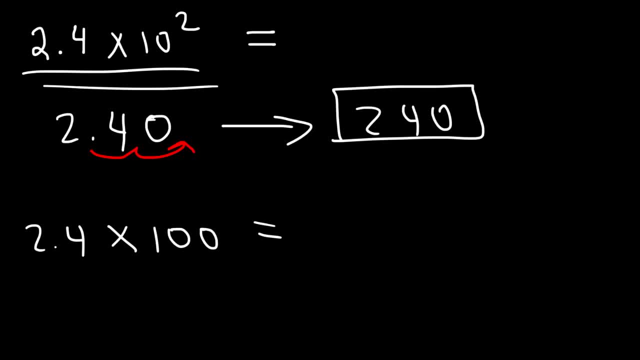 is 100.. So this really means 2.4 times 100,, which is 240.. And so you know what this expression means: 10 squared, that's 10 times 10,, which is 100.. So this really means 2.4 times 100,, which is 240.. 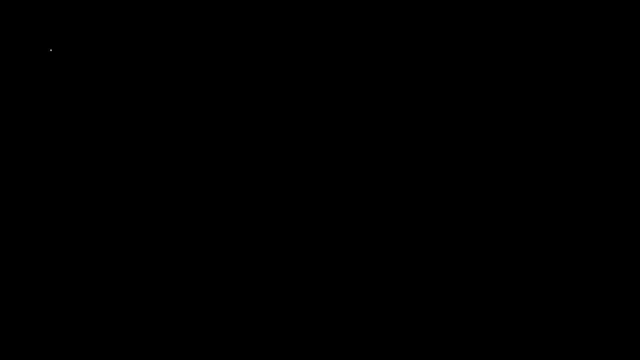 So you could see it that way. if you want to as well, Let's try this example: 3.56 times 10 to the third power. So we need to move the decimal 3 units to the right. So this is 1,, 2,, 3.. 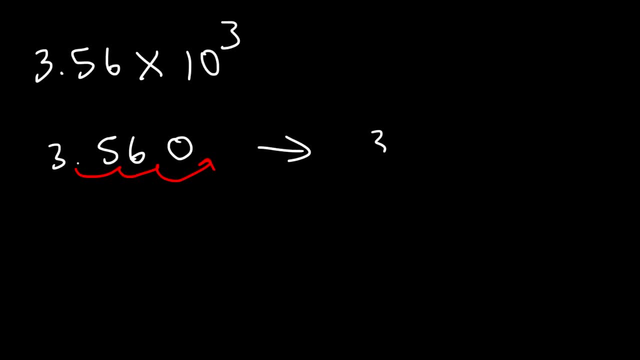 So we need to add another zero. So therefore this is going to be 3560.. So 10 to the third means that, well, 10 times 10 times 10, that's 1000.. So that's 3 zeros. 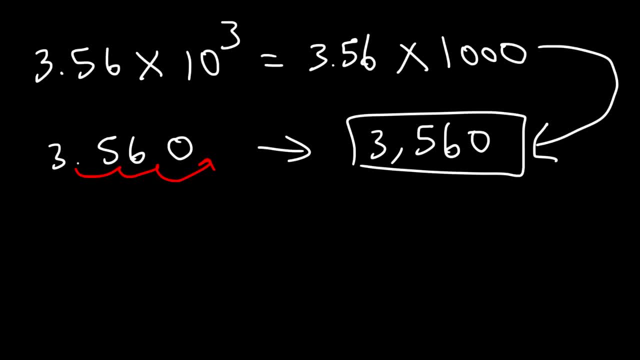 And 3.56 times 1000 is 3560.. Go ahead and try these two examples: 4.27 times 10 to the 5. And also 3.96 times 10 to the 7.. So let's start with this one: 4.27.. 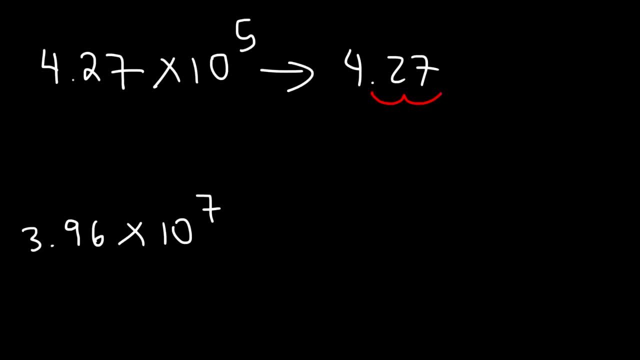 Let's move the decimal point 5 units to the right, So that's 2, 3,, 4,, 5.. So we need to add 3 zeros. So this is going to be 4, 2, 7, 0, 0, 0.. 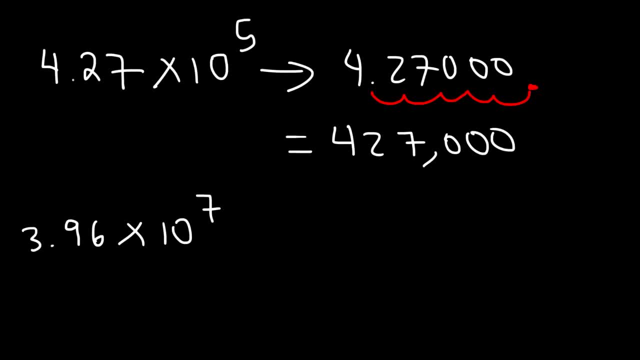 Or 427,000.. 10 to the 5th is basically 100,000.. So 100,000 times 4.27, that's 427,000.. Now let's try this one. So we have 3.96 and we need to move the decimal point 7 units to the right. 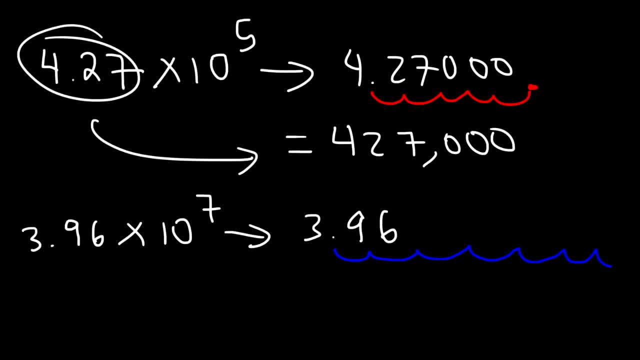 So 1,, 2,, 3,, 4,, 5.. So that's 1,, 2,, 3,, 4,, 5.. 5,, 6,, 7. And so we need to add 5 zeros. 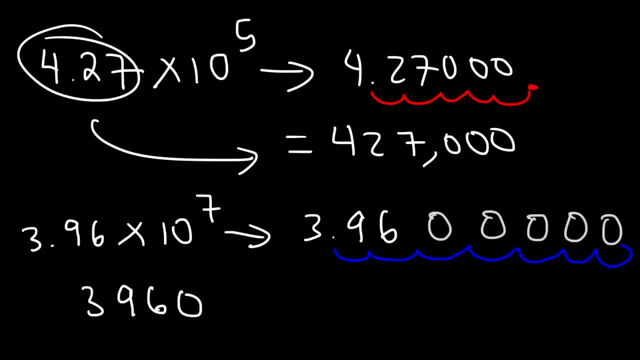 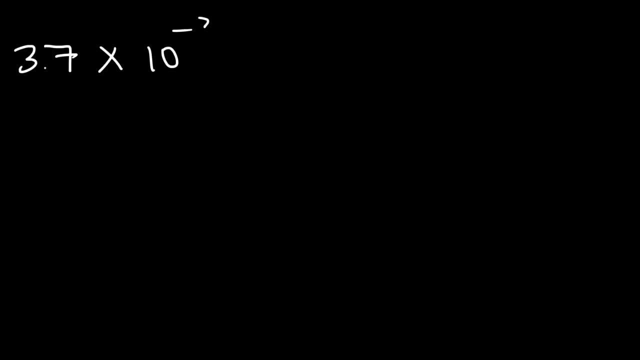 So the answer is going to be 39600000.. So that's 39,600,000.. Now let's work on some examples with negative exponents. So a negative exponent, A negative exponent, A negative exponent associated with a small number. So this time we need to move to the left. 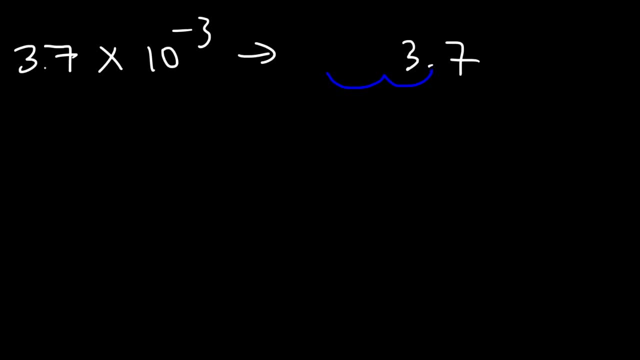 So let's move three spaces to the left: 1,, 2, 3.. So we need to add two zeros. So therefore this is going to be 0.0037.. Let's try this example: 4.16 times 10 to the negative 5.. 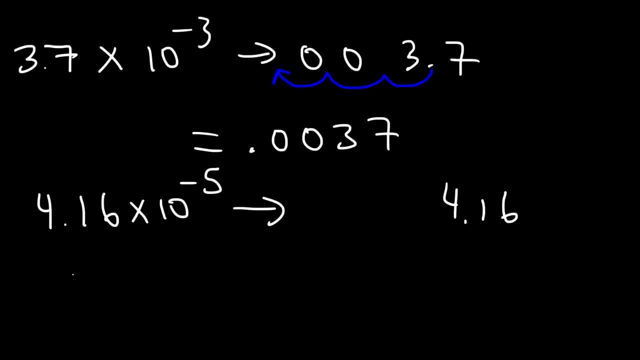 So we need to move five spaces to the left: 1, 2,, 3,, 4, 5.. So this is going to be 0.000416.. Now let's work on a mixed review. Go ahead and convert the. 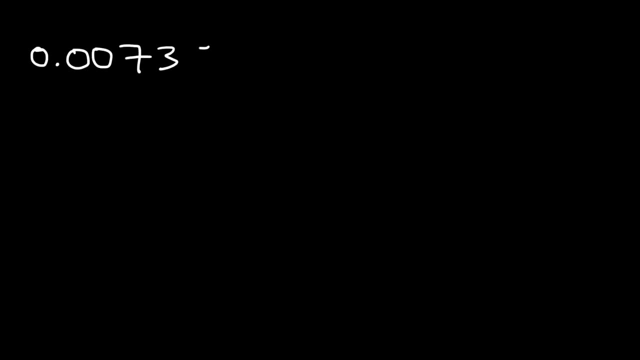 numbers into scientific notation. Let's see if you remember how to do that. So the first one is a small number, so it's going to be associated with a negative exponent. We need to move the decimal point between the 7 and the 3, between the first two. 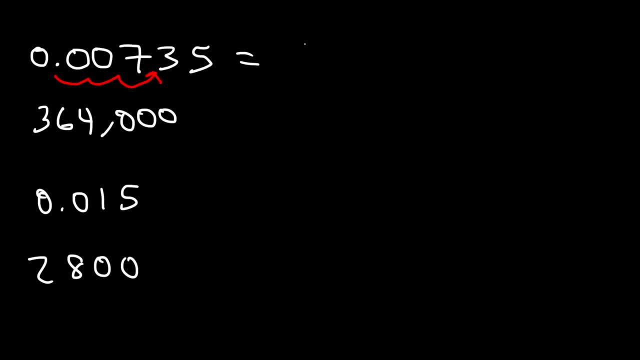 non-zero numbers. So since we move it three units to the right, it's going to be 7.35 times 10 to the negative 3.. Now let's move on to the next example. We have a large number and we need to put the decimal between the first two non-zero numbers, between the 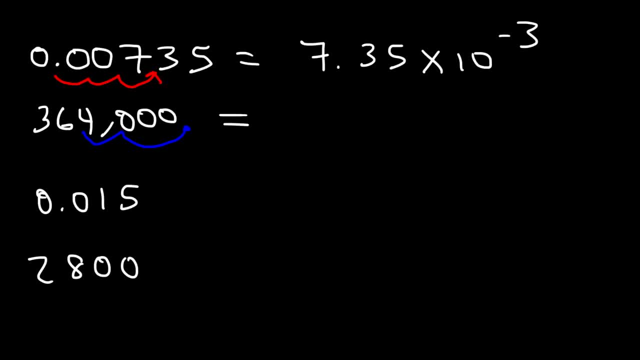 3 and 6.. So we're going to move it 3,, 4, 5 spaces to the left. So this is going to be 3.64 times 10 to the positive 5, since we have a large number. Now the next example. 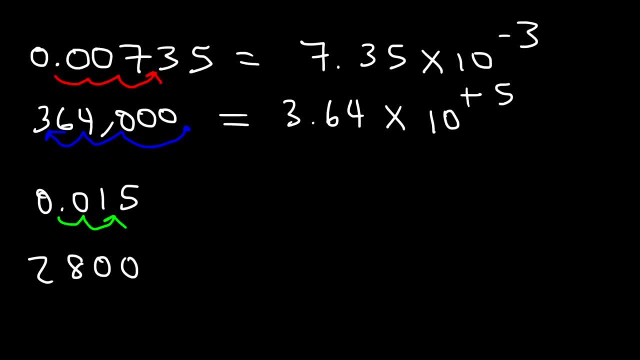 is a small number and we only need to move it two spaces to the left, So this is going to be 1.5 times 10 to the minus 2.. And for the last example, we have a large number and we're going to move it three spaces to the left, So this is going to be 2.8 times. 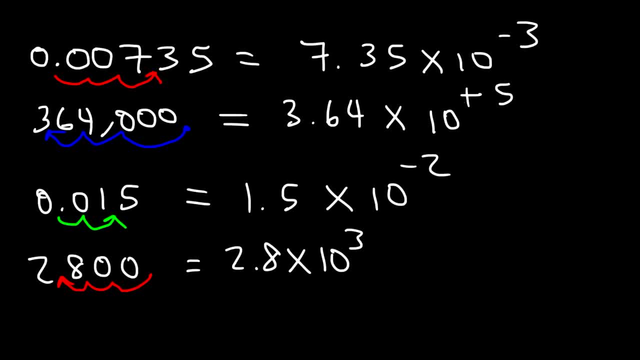 10 to the 3.. So keep that in mind. Anytime you have positive exponents, it always will be associated with large numbers, And small numbers that are between 0 and 1 are associated with negative exponents. That will help you to determine which direction you need to move. 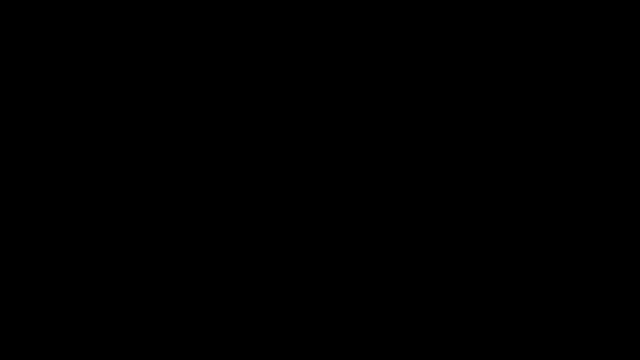 the decimal point. So let's try some more. Let's try some more examples: 1.8 times 10 to the minus 3, 4.1 times 10 to the 2, 1.2 times 10 to the negative 5, and 2.7 times 10 to the 4.. So let's convert this to standard. 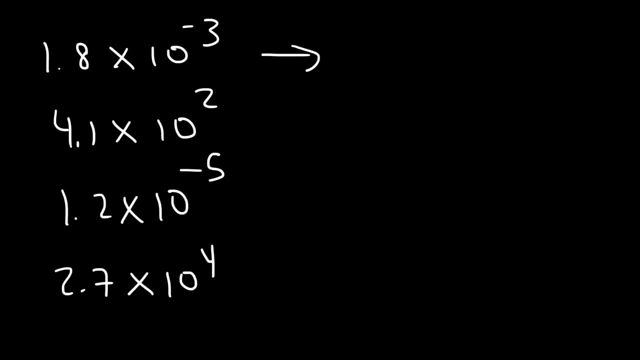 notation. So let's start with the first example. Should we move the decimal point to the left or to the right? This is particularly useful if you need to convert it from scientific notation to standard form. So let's start with the first example. 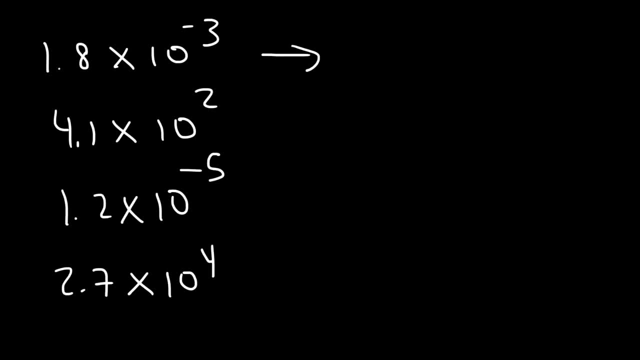 Since we have a large number, we're going to move it three spaces to the left, So we're going to have a negative exponent. We need a small number, So we've got to move it to the left: 1,, 2, 3.. So we're going to fill these spaces with zeros. So therefore this: 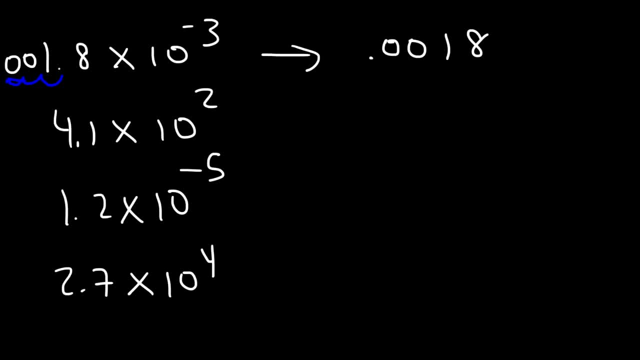 is going to be 0.0018.. Now for the next example. we have a positive exponent, So that's associated with a large number. Therefore, we need to move the decimal point to the right two spaces. So we're going to add a zero here. Therefore that's going to be 410.. 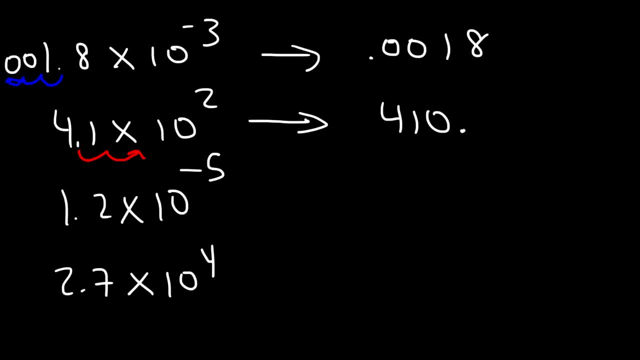 Now for the next example. we need to move it to the left: 1,, 2,, 3,, 4, 5.. So, therefore, that's going to be 0.00 0012.. Now there are surrender beings. Therefore, we need: